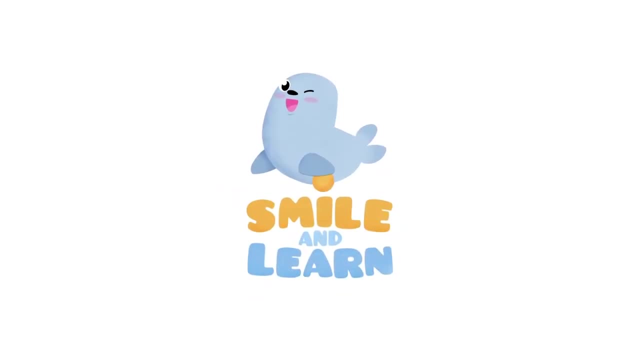 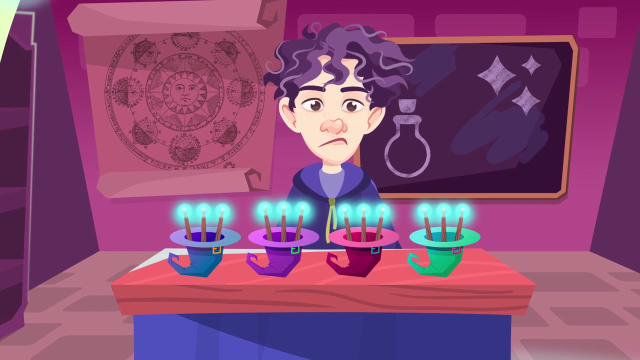 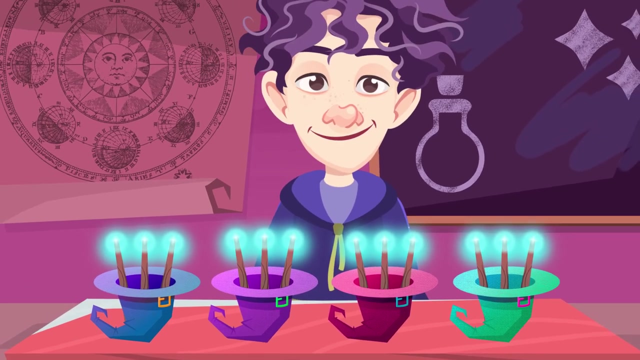 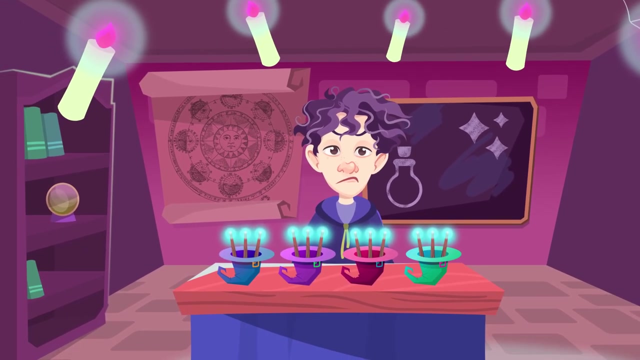 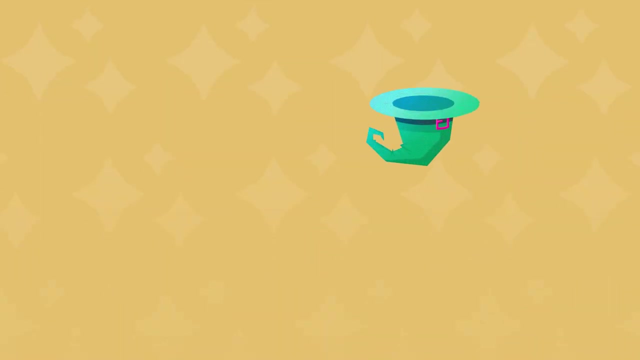 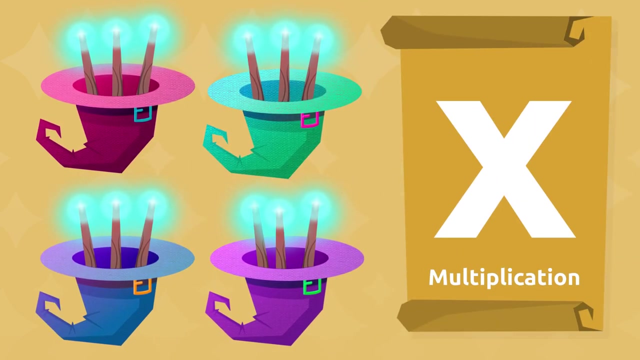 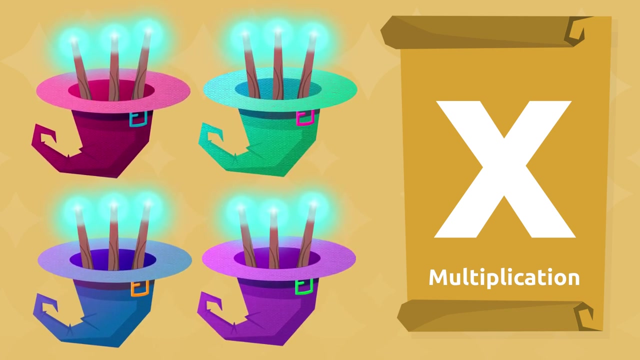 Smile and Learn Wizard. my friend, together we're going to count all these magic wands thanks to the math operation of multiplication. Multiplying is like adding the same number several times. It's a math operation. you're going to be doing a lot, day after day. 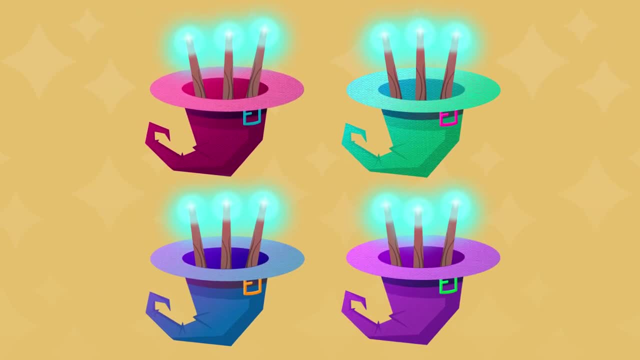 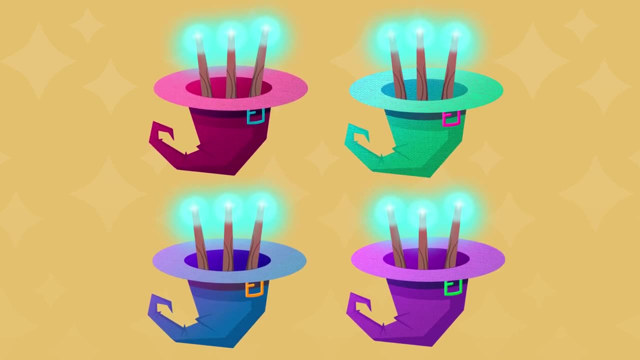 It's easy peasy, You'll see. As you can see, there are four hats and three wands into each one of them. In what way could we work out how many wands there are All together? We can try two ways. 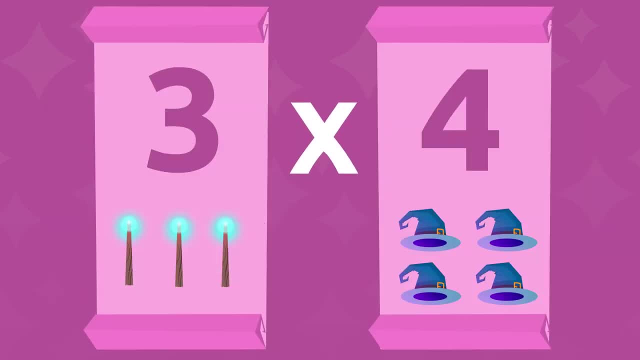 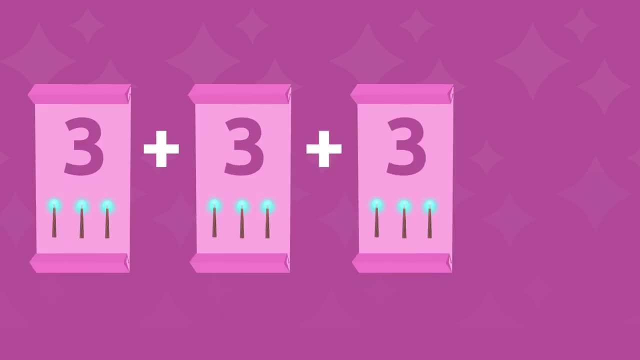 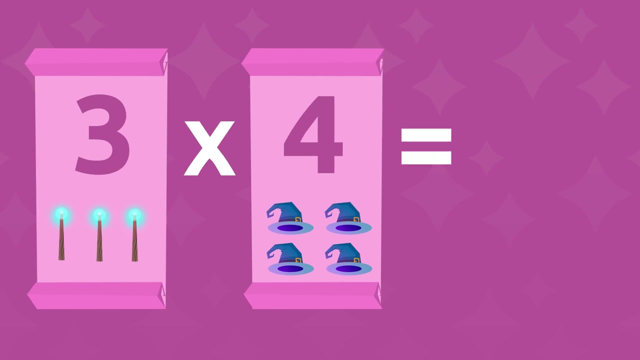 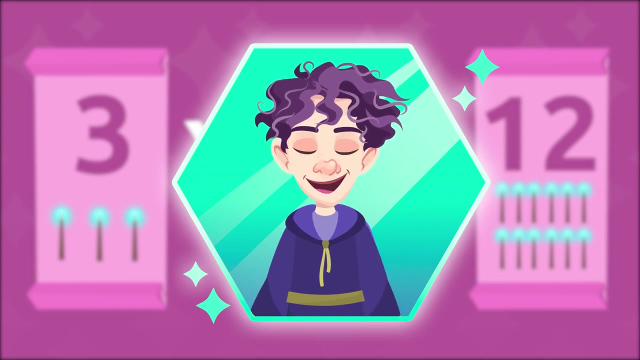 Adding up or multiplying Meaning. we can calculate it like this: Three wands plus three more wands plus three more plus three more, Or three wands by four hats. Both ways will give us the same result: The number twelve. So to multiply is to add up several times. 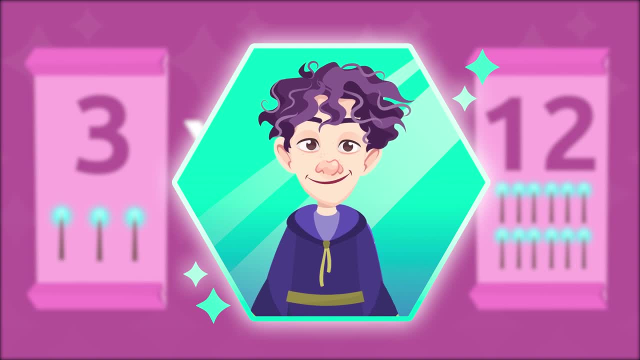 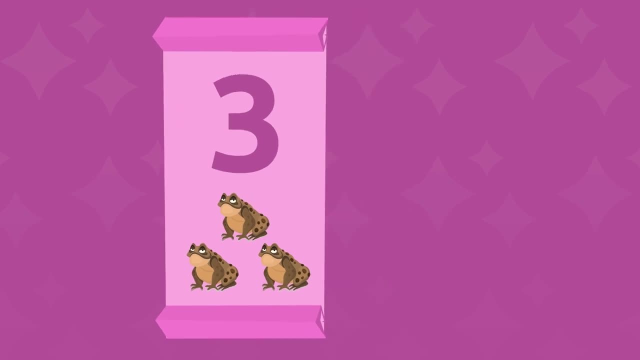 The same numbers. right, That's it. Let's look at another example. Imagine you need to buy three toads for your magic potions class. If each toad costs two coins, how many coins do you need to buy three of them? 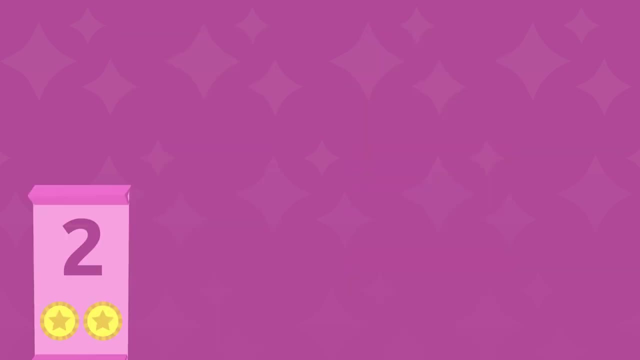 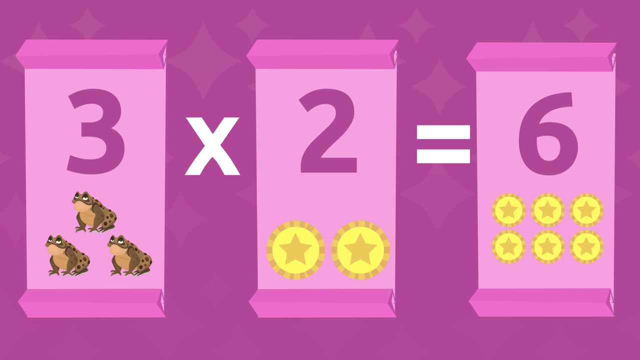 It's very simple. We can add up this way: Two coins plus two coins plus two coins, Which equals six coins. Or we can multiply Three toads by two coins, Two coins each, which equals six coins, Meaning three toads cost six coins. 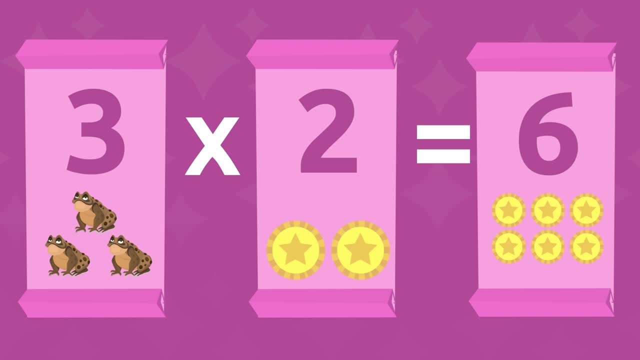 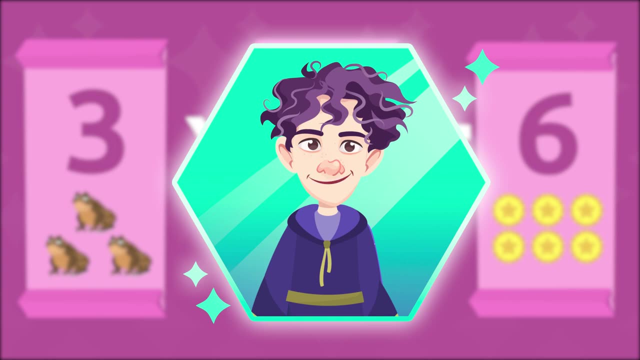 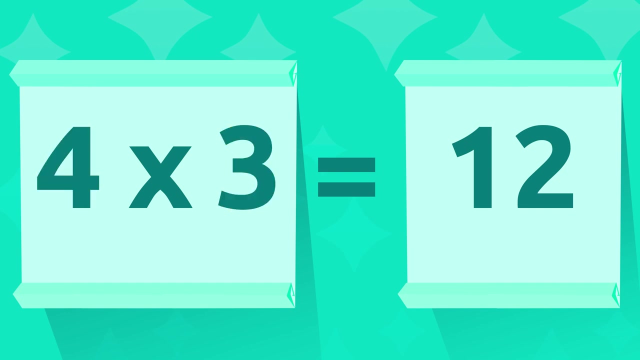 Do you see how fast you can count now that you know how to multiply? I do. It's incredible. My friends are going to be amazed. And how do you call these multiplication numbers? You mean the parts of multiplication. The numbers to be multiplied are called factors.